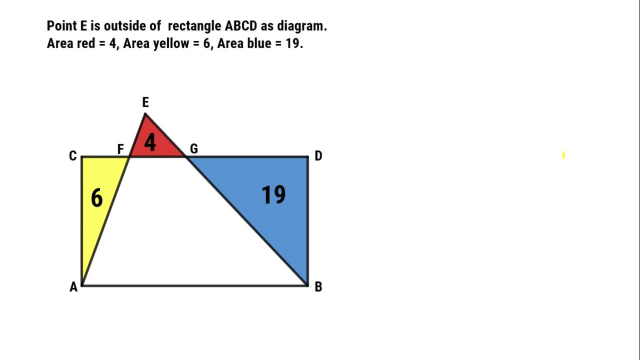 Point E is outside of rectangle ABCD. as diagram, Area red is 4 units, Area yellow is 6.. Area blue is 19.. Problem is: what's the area of rectangle ABCD? Before watching this video, you can make a try to solve this problem. 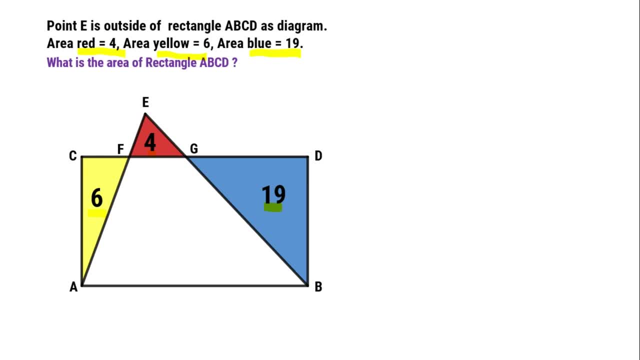 Maybe you will find something different with me. Make a parallel segment to CD through point E. Make a parallel segment to CD through point D. Make a perpendicular segment DH to it. If we move point E closer to point H, we could guess the length of FG is a constant. 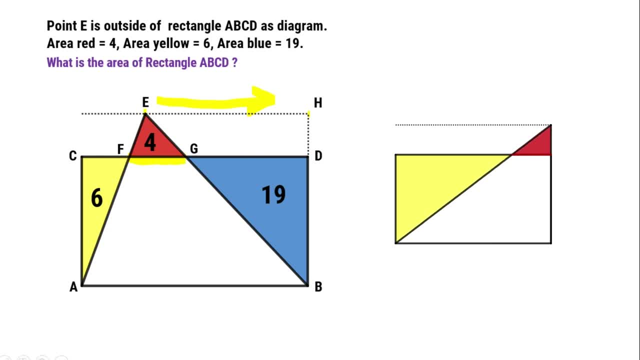 If we move point E closer to point H, we could guess the length of FG is a constant. If we move point E closer to point H, we could guess the length of FG is a constant. Connect AH, Intersect CD in point J. 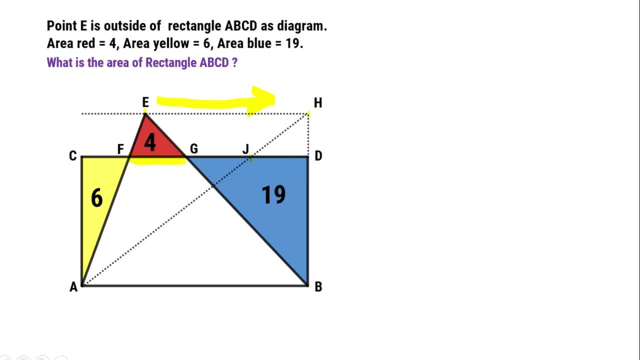 Now let's prove FG equal to JD, FG over AB, FG over AB, Equal to HD over HB, Equal to HD over HB, Equal to HD over HB. Because triangle EFG is similar to triangle EAB. Because triangle EFG is similar to triangle EAB. 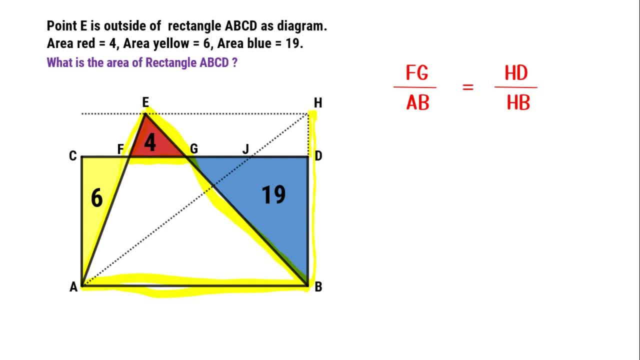 HD is the height of triangle EFG. JD over AB, Also equal to HD over HB. Because triangle HJD is similar to triangle HAB, we can get fg equals to jd. So the area of triangle hjd equals to area of triangle efg is 4 units. 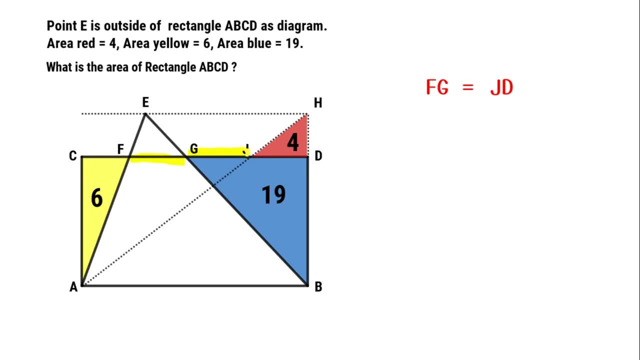 fg plus gj equals to gj plus jd. We can get fj equals to gd. So the area of triangle afj is equal to 19 units. Triangle jdh similar to triangle jc. Use the principle of proportional area theorem. We can get jd squared over jc. squared equals to 4.. 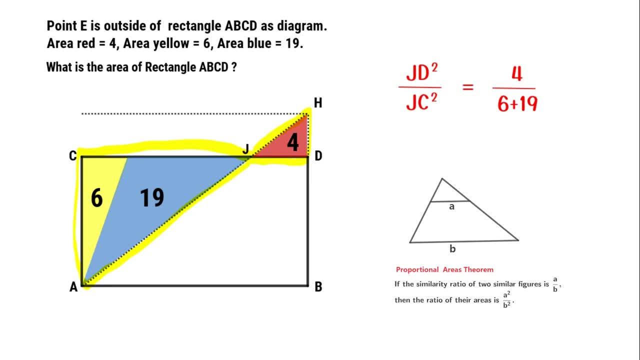 Over 6 plus 19.. jd over jc is 2 over 5.. Connect ad Use the principle of same height of two triangles. We can get area triangle ajd over area acj. Area triangle of ajd over 25 equals 2 over 5.. 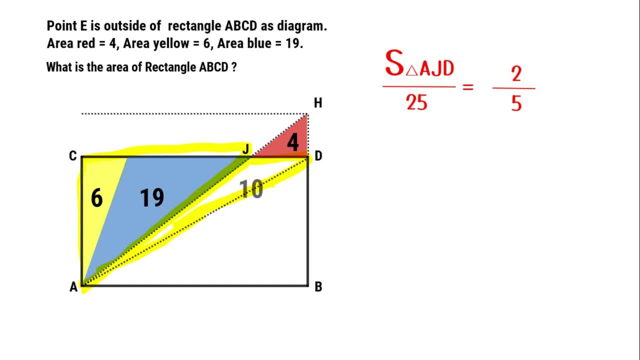 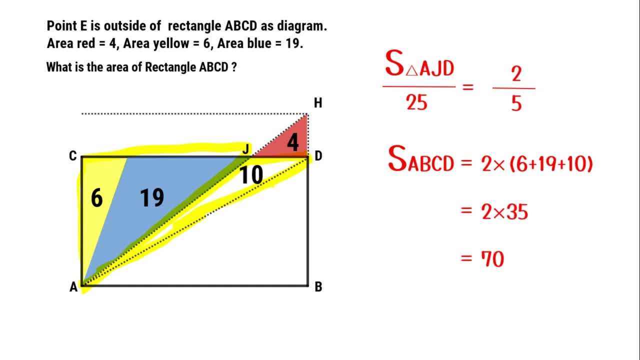 plus 10 is 70 units. Thank you for watching this video. Please don't forget to thumbs up and click the subscribe button. if you don't subscribe my channel now, Turn the bell on. You will not miss my future videos. See you next time.